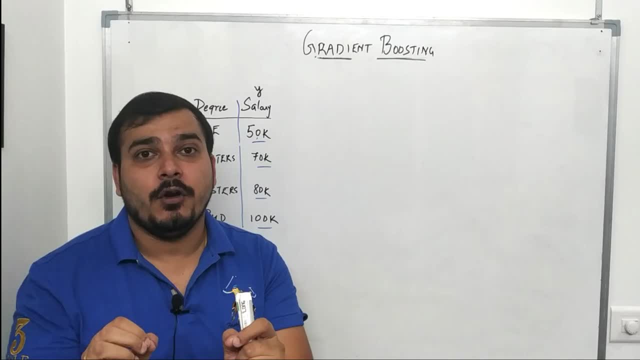 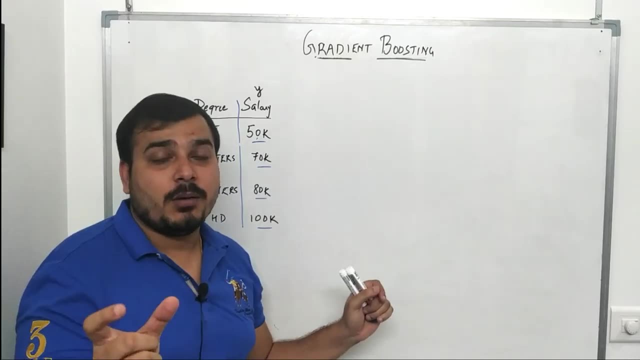 working of this gradient boosting, because it will be definitely very, very helpful when you are actually going for the interviews Right in the third part- and again, why first and second part? it is with respect to regression problem statement. I'll be discussing and then I'll be going ahead. 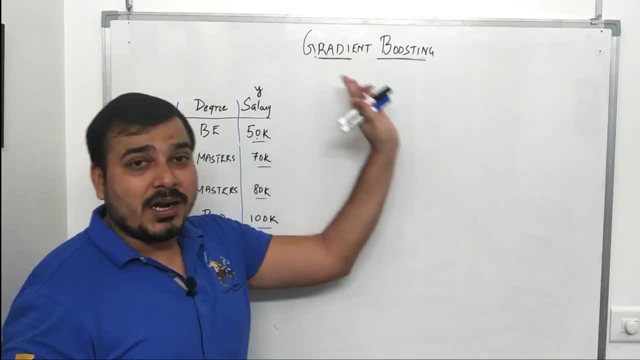 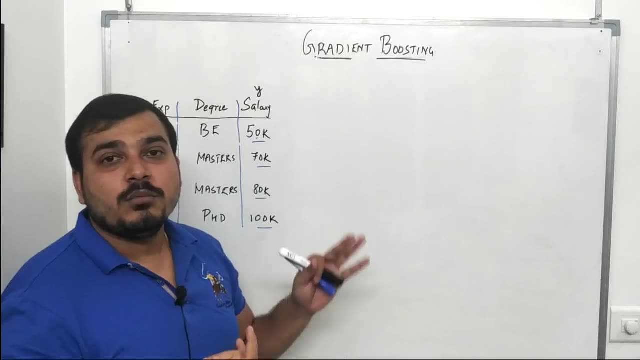 with classification problem statement And with respect to this guys, you need to understand this very properly because this is one of the you know when I talk about all the ensemble techniques like random forest data boost, gradient boosting, extreme gradient boosting. these are one of the best algorithms that are used to solve a lot of problem statements, So it is better that. 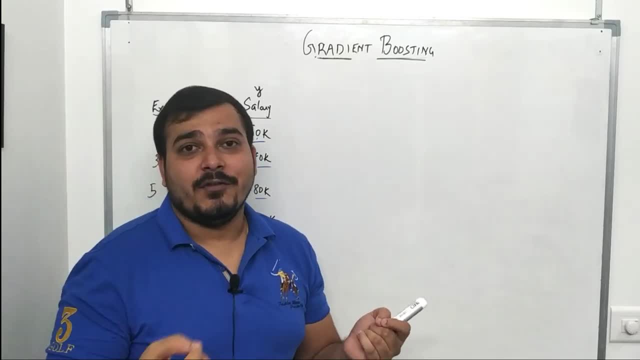 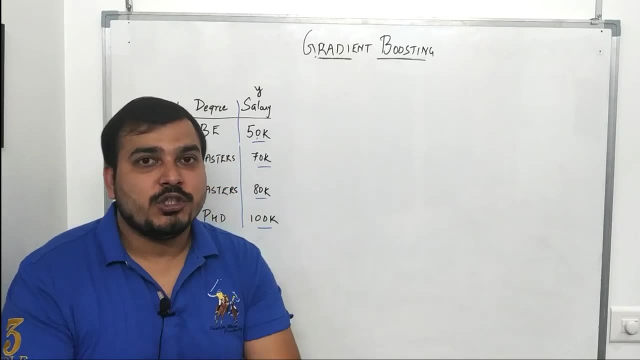 you understand this, and this is also one of the most favorite interview topic for the interviewers itself. So let us go ahead and try to understand. how does gradient boosting actually work? Now, with respect to gradient boosting guys, this is a boosting technique and if you have seen my complete 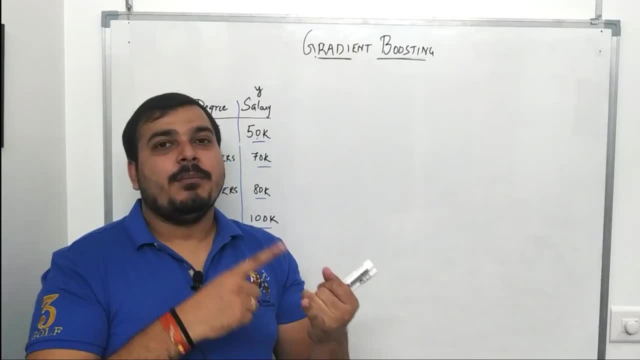 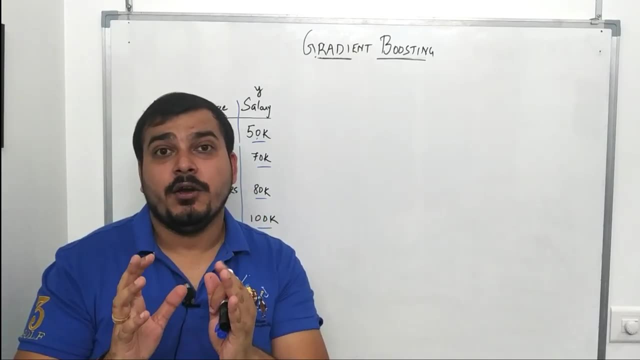 machine learning playlist. I've discussed about both bagging and boosting technique. In bagging technique, I've discussed about random forest, and in boosting, I've also discussed about gradient boosting. Now, before going ahead with respect to this particular video, you need to have a proper understanding of decision trees. How does decision tree actually work? Okay, so if you 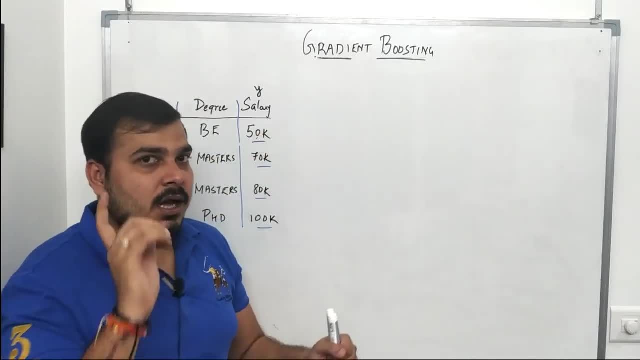 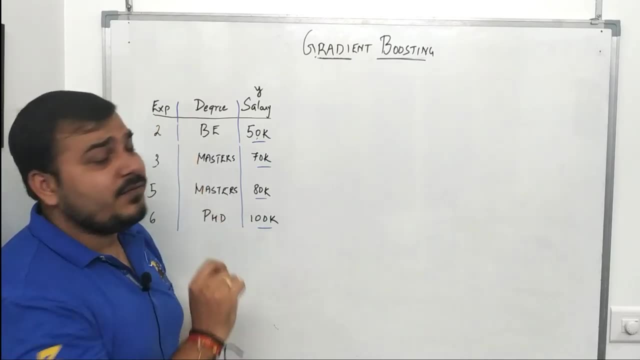 if you don't know about this, guys, it will be very difficult for you to understand this. Now let us go ahead and try to understand. how does the gradient boosting work? Okay, now I have a data set. in my independent feature. I have experience and degree. My dependent feature is having salary. Now this is 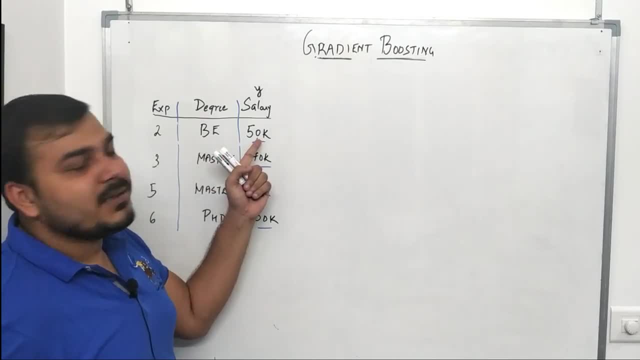 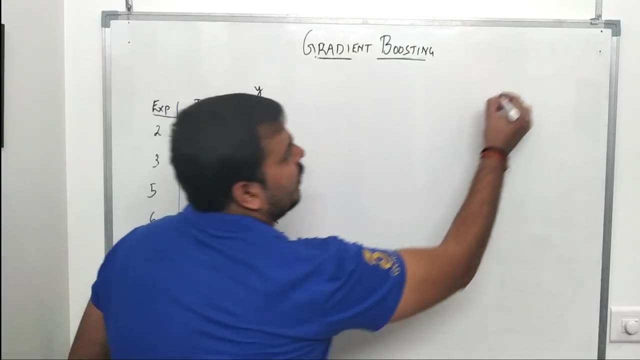 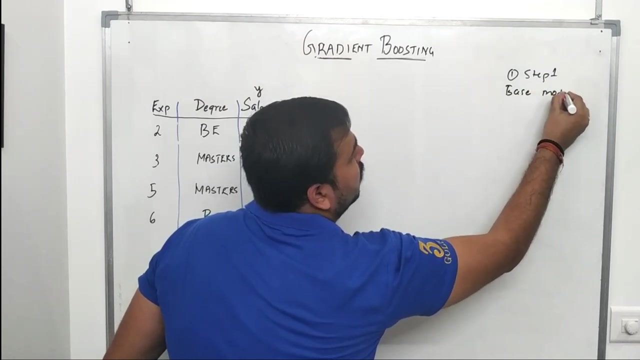 my input features like: experience is two years, degree is b, then this is my salary and similarly, right now, what is the first step in decision tree? So let me just write it down. My first step is to compute the base model which will give me one output. which will give me one output. Now what? 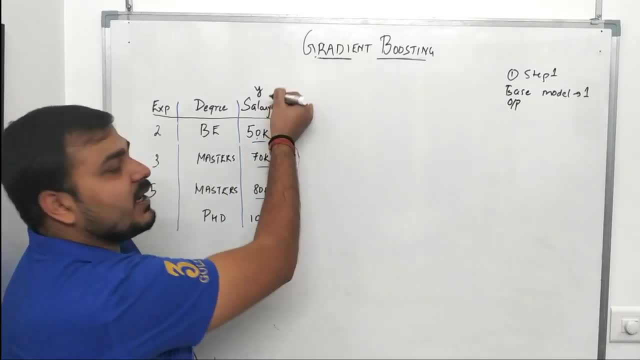 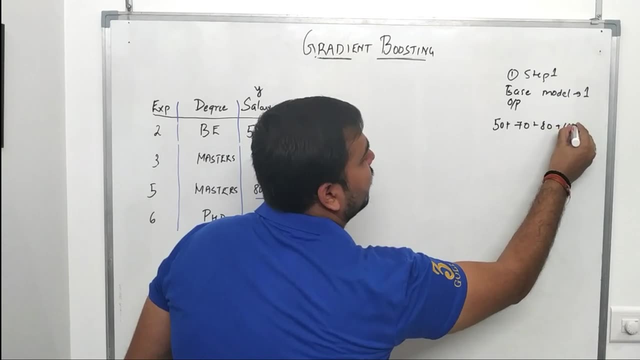 will be this output. this output will be the average of all these particular values, average of all this salary. So if I try to compute the average- 50 plus 70 plus 80 plus 100 divided by 4, right now, if I try to find out the average, the approximate value that I'm going to take, 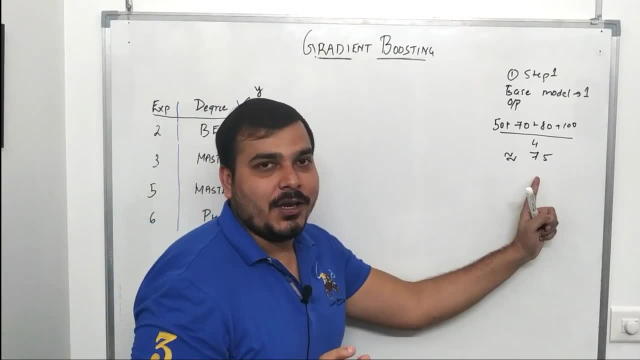 take is 75, guys. Okay, now don't tell me, Krish, you have not written the right value, You have not computed it rightly. Don't do that. I have just taken an example. Okay, 75k. Okay. 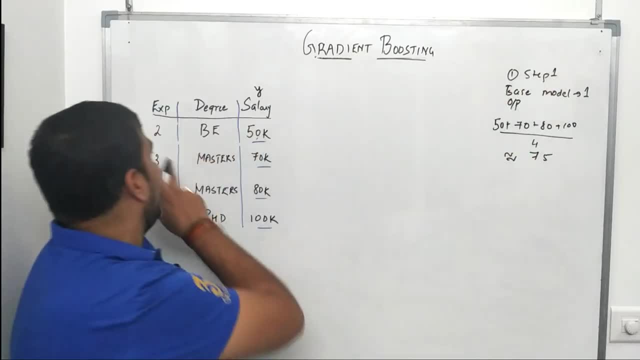 so this is my first base model And remember, whenever I give my training data set, the output will be only 75.. Pretty much clear, right? So let me write it down over here. Okay, this is my y hat. y hat is basically my predicted value. So I'll be having 75,, 75,, 75,, 75.. Okay, pretty much simple. 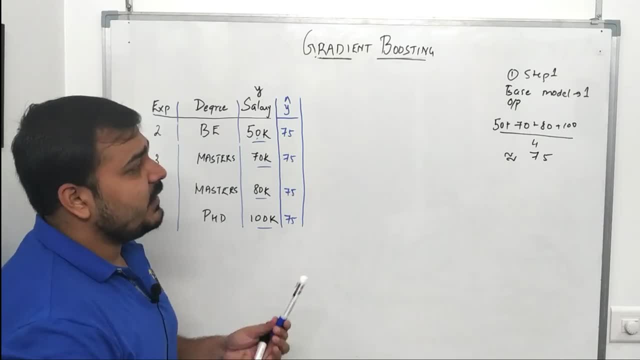 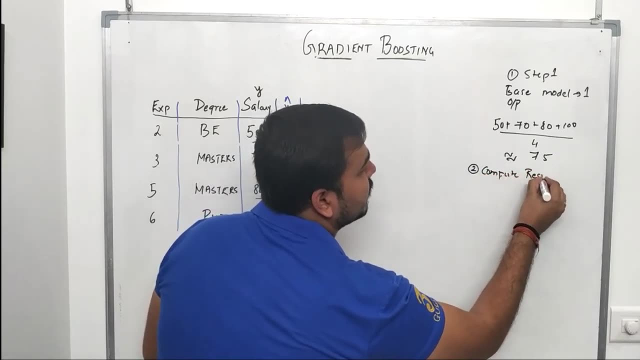 Done first step. Okay, now in the second step, in the second step, we will be computing, compute residuals. Residuals basically means errors, Okay, errors, or I can also call this as pseudo residual. I'll tell you why. pseudo residual guys? Because, understand, in order to 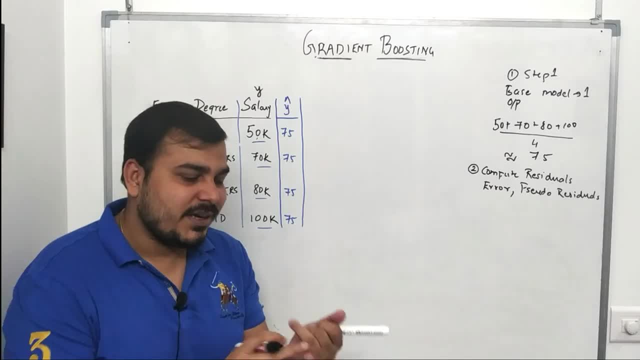 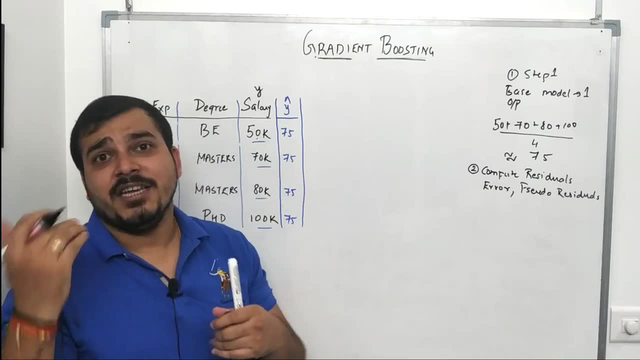 compute errors. we basically use a loss function. You know, in regression you have different kind of loss function like mean squared error, root mean squared error. We have loss functions in classification like log loss. we have hinge loss and many more losses right? So based on that, 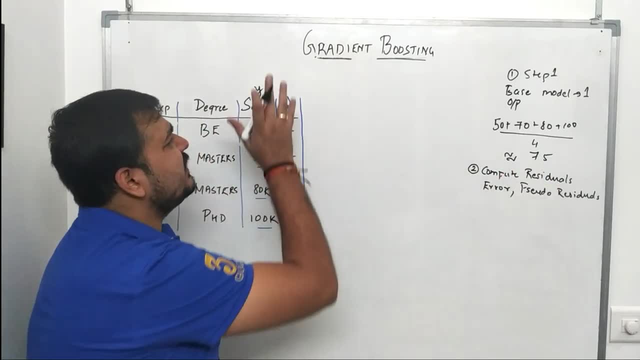 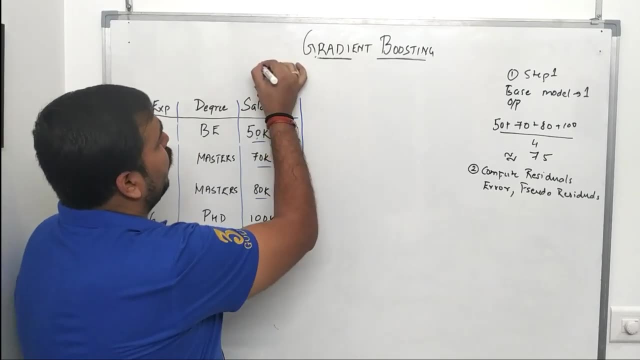 we'll try to compute the residual errors. Now, in this case, we'll use a simple- you know we'll be using a simple loss function. just consider this Here: my loss will actually be what I'll try to do in order to compute the residual. I will just subtract my actual value with the prediction value. 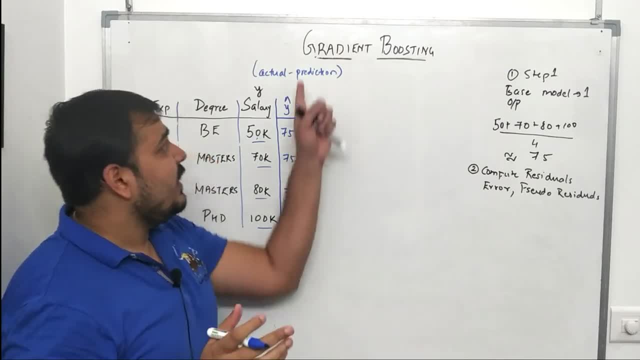 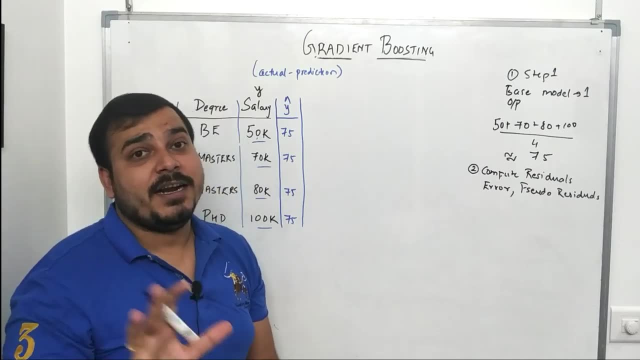 just for an example, Guys, here you don't tell me that why I'm not taking squared. just to show you an example, Because in the next video, where I'll be discussing about the pseudo algorithm, there I'll be telling you about different kinds of loss functions And there I'll be using the exact. 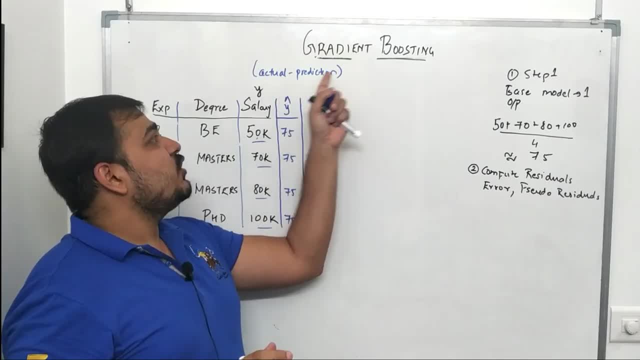 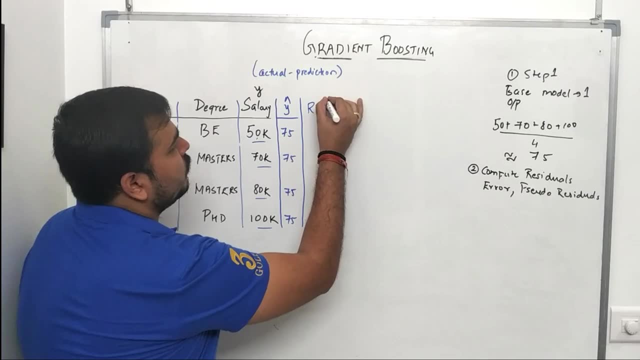 formula. In this case, what I'm doing, I'm just trying to subtract the actual value with the prediction value. Okay, now this: initially, when I'm subtracting this, I'll write a new column that is my R1.. So this is basically my residual one. Now, with respect to this, 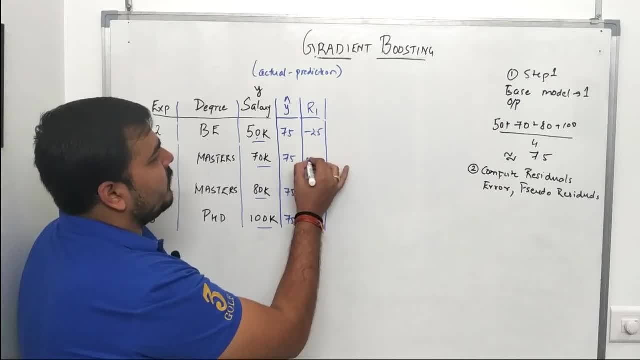 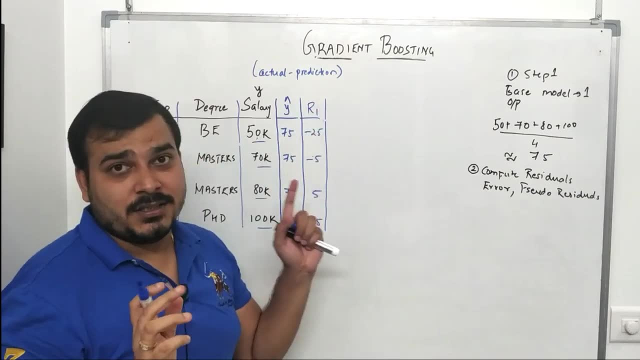 guys, if I subtract 50 minus 75, it is nothing but minus 25.. This is minus 75.. Okay, now 25, this is minus five plus five and 25.. I understand, this is my R1, my residuals, my errors. 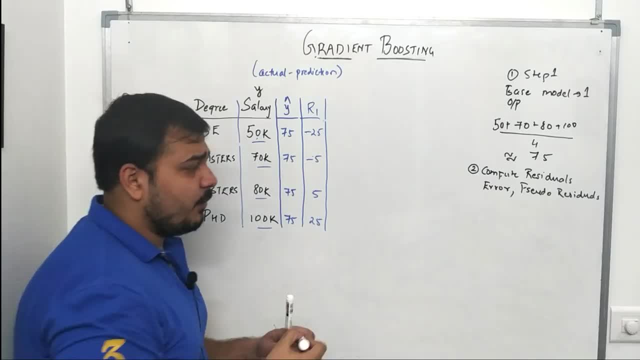 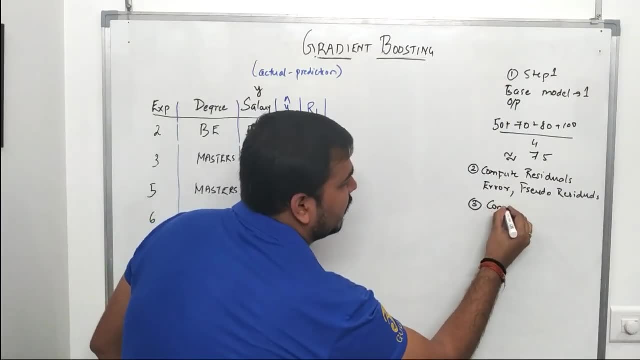 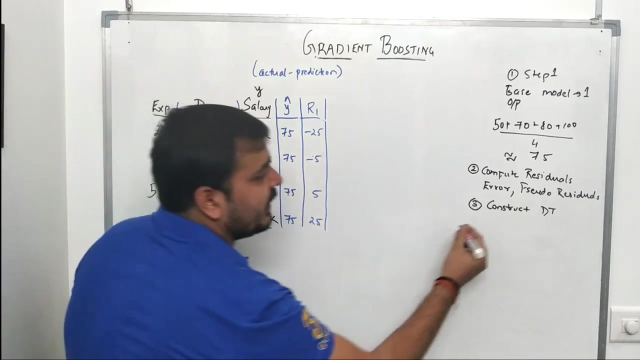 okay, in the first phase. Now, third thing, guys, third, very important thing: Now, after this base model, I will add one decision tree sequentially. So I'll construct a decision tree Now, in this decision tree, in this decision tree, my input will be my experience and degree. Okay, this is. 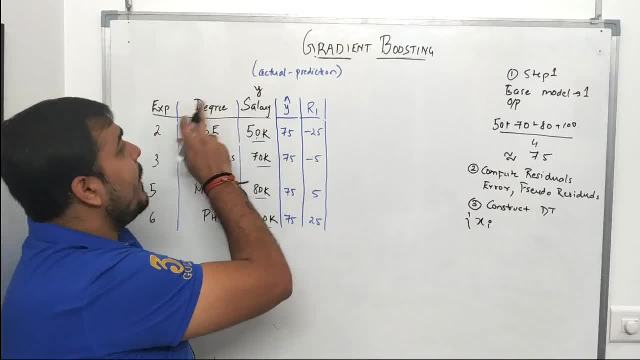 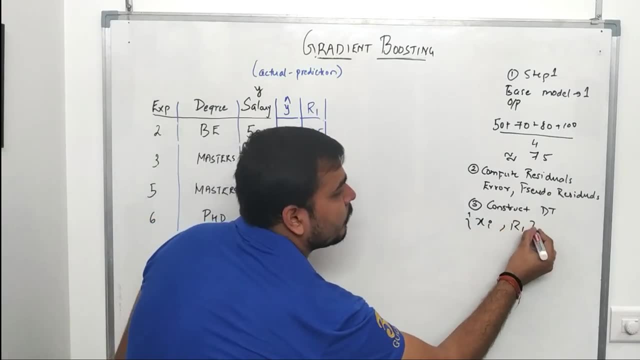 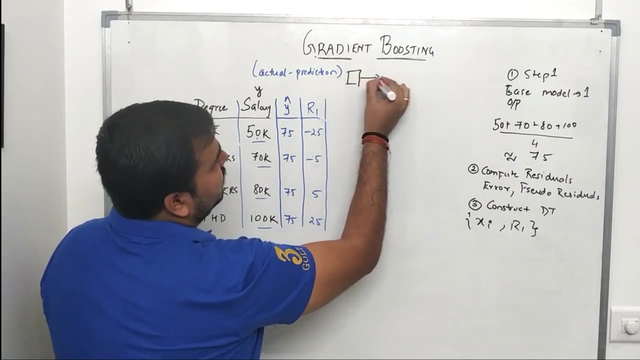 my Xi. that is same input, like experience and degree. Now I'll add one decision tree sequentially, But my output value, my dependent feature, will not be salary, it will be this residual error R1.. Okay, in this it will be a residual error R1.. So what I've done, this is my base model. After this, 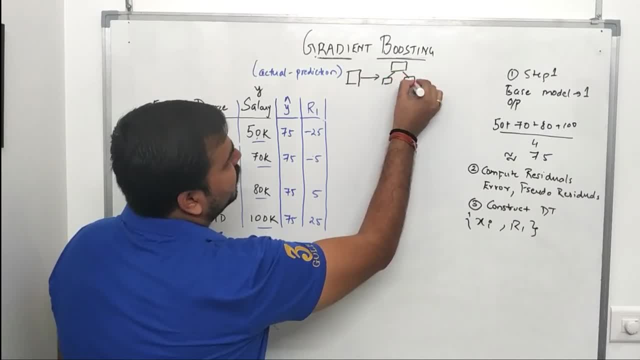 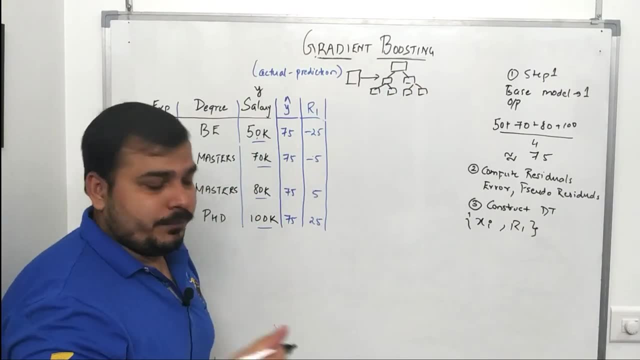 I've added a decision tree. I've trained with the data where I have independent features And my output is basically my residual. So I have trained this decision tree Right Now. one important thing: okay, When I've trained this data and when I've trained my decision tree, I've trained my 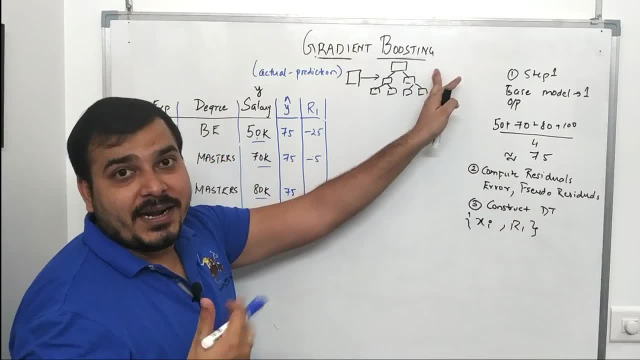 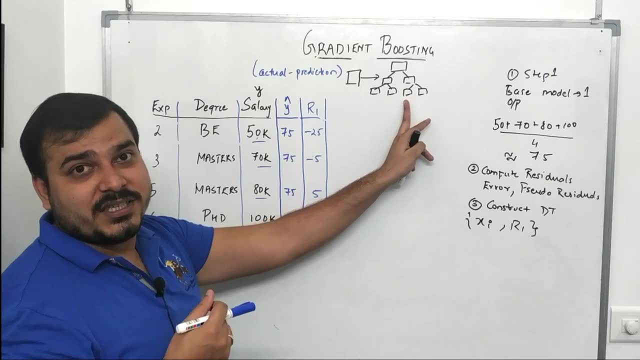 decision tree with this data. obviously my decision tree will predict the output of the residuals, only right. So if I pass my independent feature once again to this decision tree, okay, once again to this decision tree- I will be having my R2 feature, Suppose my R2, residual 2, that is. 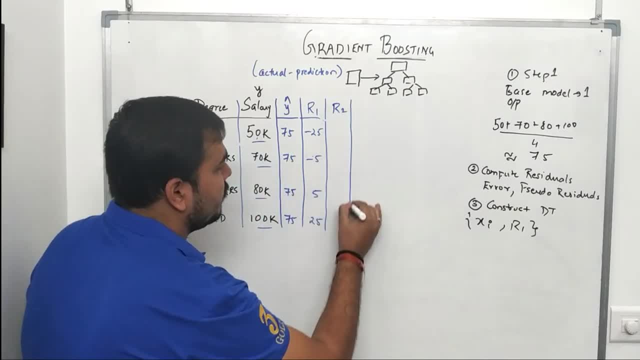 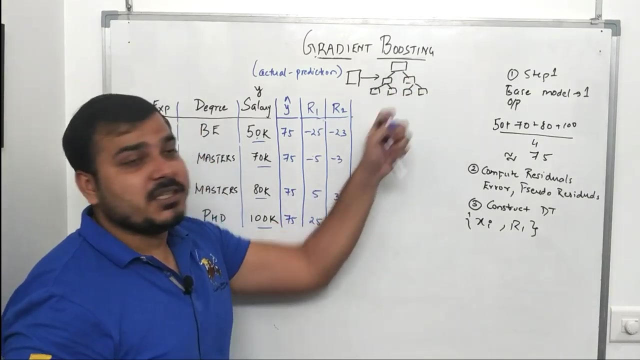 coming out after passing. this independent feature is somewhere like this: Suppose I get minus 23,, minus 3.. Okay. Suppose I get 3 and this is suppose 20.. Suppose I get this kind of residuals right, Residuals that I'm actually getting the output right, output from this decision tree. Now still. 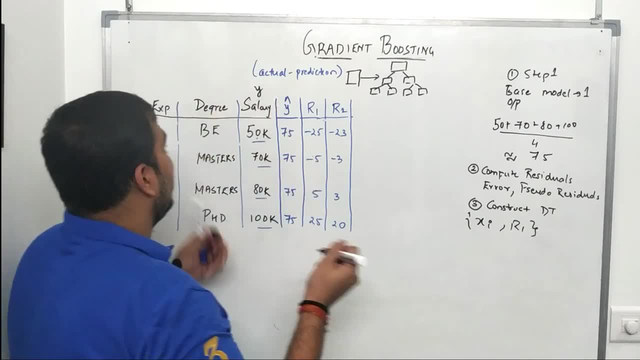 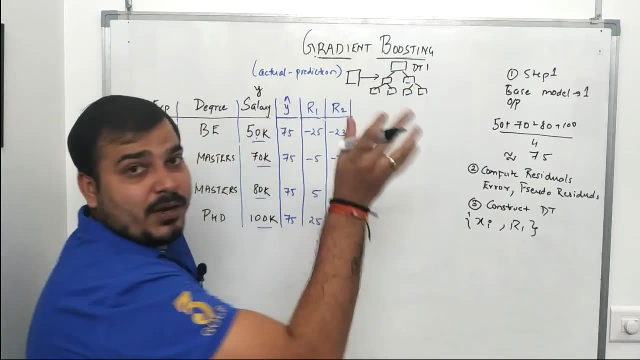 I don't know how to compute the salary, So let us see how to compute the salary Now. suppose I pass this particular value to this two models. one is the base model and one is to the decision tree, one, okay, which is attached sequentially. then what is the output I'll get? 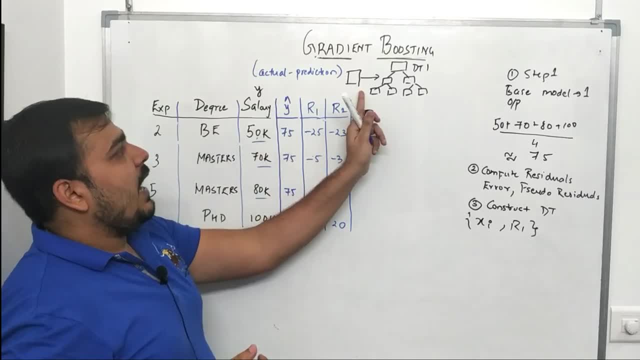 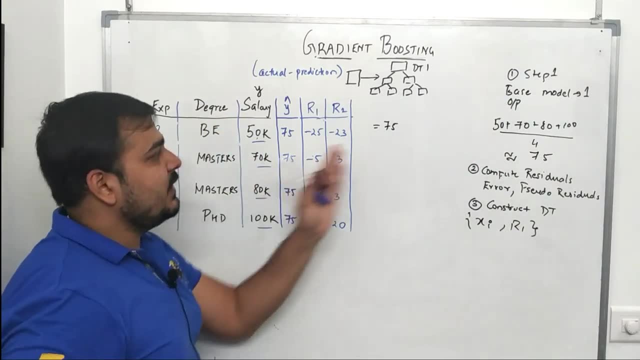 So whenever I pass to the base model for the first record, I will definitely get 75, right, I'll be getting 75, because always remember my base model, whatever records I pass, it will give me 75. So, after the base model, I've got the value of 75.. Now, with respect to decision tree one, I will be 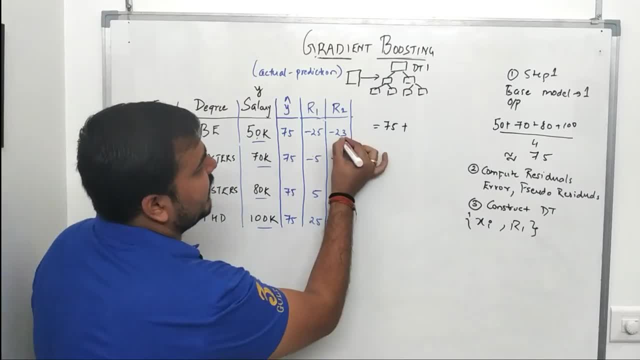 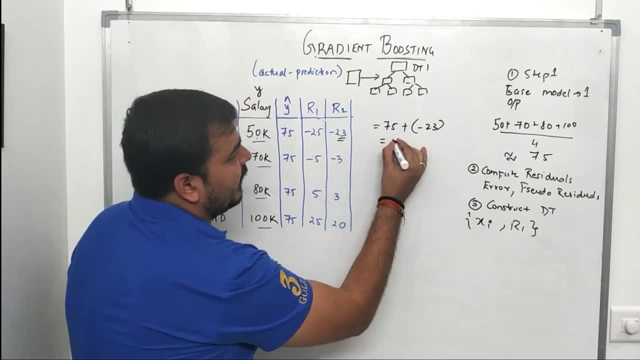 getting some residual value right, Some residual values, Now. suppose in this case I will be getting a residual value of minus 23 for this record, for the first record right, for the first record. And now, if I try to subtract 75 minus 23,, what it will be, it will be somewhere around 52,. 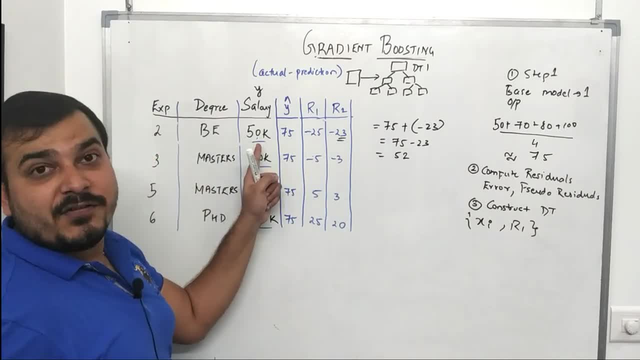 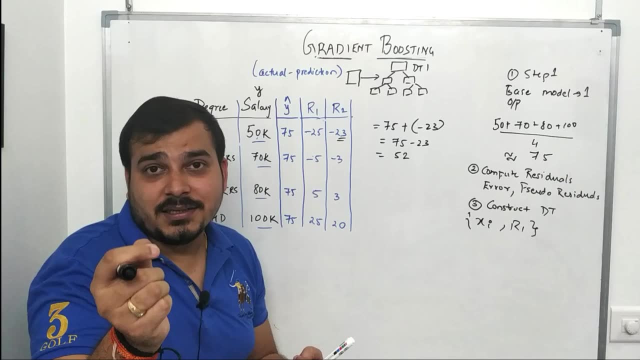 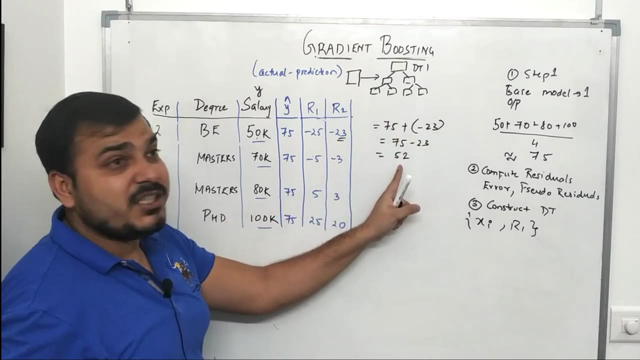 right Now, this 52 and my actual value, 50, is very, very much near. So do we think that this model is going to be the best? The answer is, guys, no, Understand this is overfitting problem Here, within my decision tree one, I'm able to get a value which is very, very near to the salary. 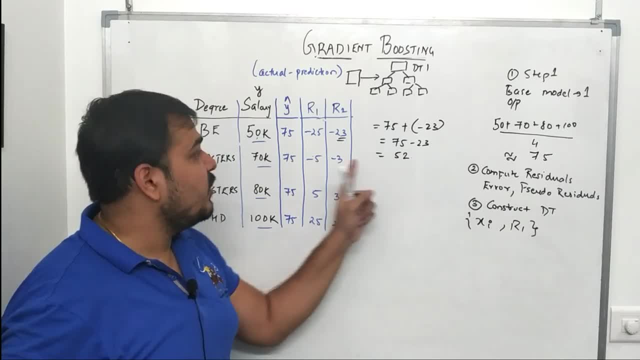 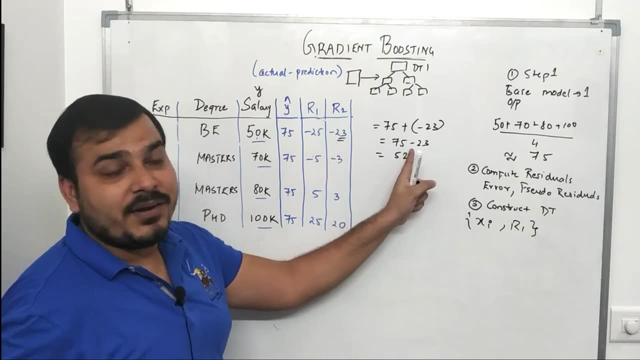 right, This is an overfitting problem altogether, right? Suppose if I had my residual 2 as 20, at that time, 75 minus- sorry, if I had like, minus 25, I would have got. 75 minus 25 is equal to 50,. 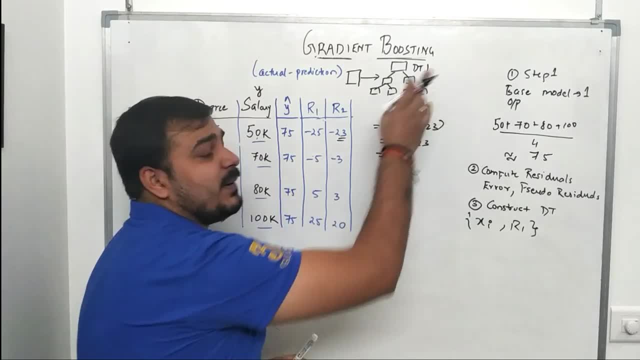 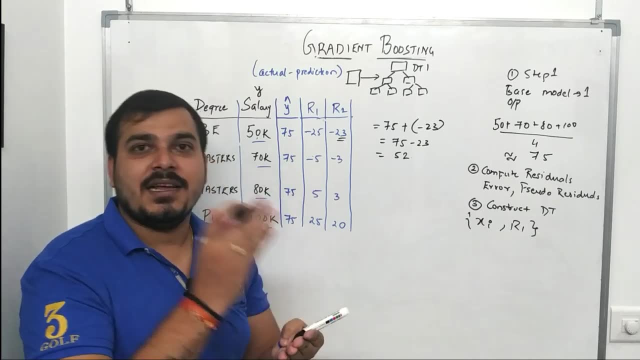 right, Which is pretty much bad. right Because, understand, with respect to decision trees, with respect to a model that we create, with respect to any models that we create, we should have a generalized model which has low variance and low bias. Okay now, in this case, 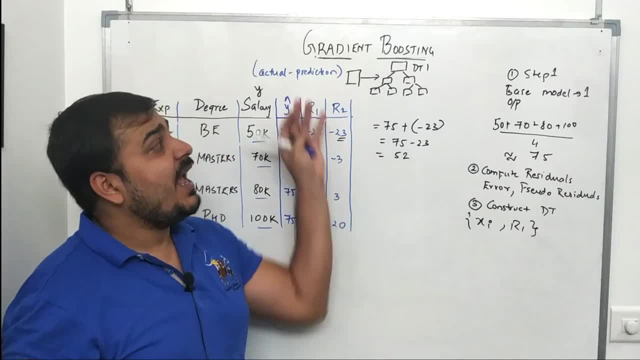 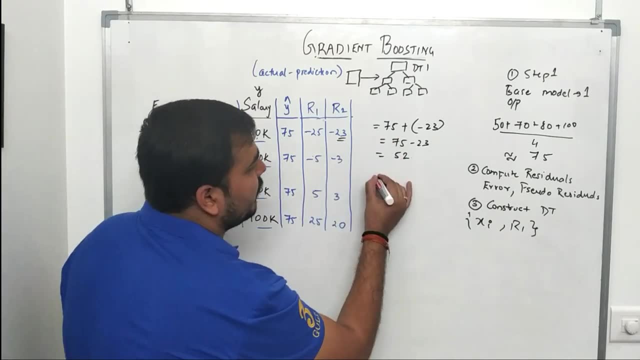 I'm having low bias but high variance, because when I get my new test data, definitely this value will be a little bit bigger, you know, for my new test data. So for that, to prevent this, what we'll do is that when we are adding this right, we will be adding a learning rate and then 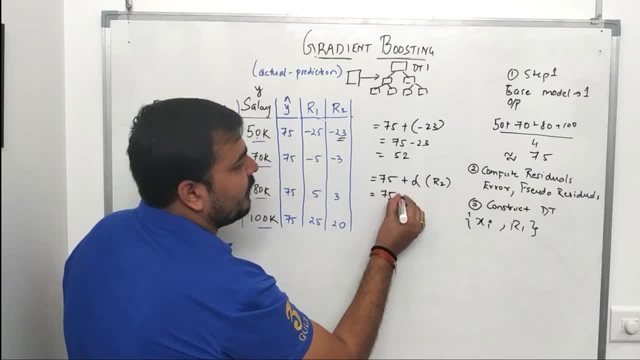 we'll be adding your R2 value the residual value. So if I write and this alpha or learning rate, like, okay, suppose I take it as point one, this residual value will be minus 23.. So I have 75 minus point two, three, sorry, it will be 2.3.. Okay, 2.3.. And here I'm getting the value of 73.7.. 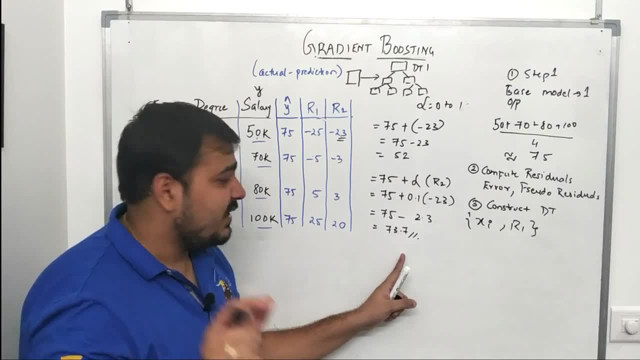 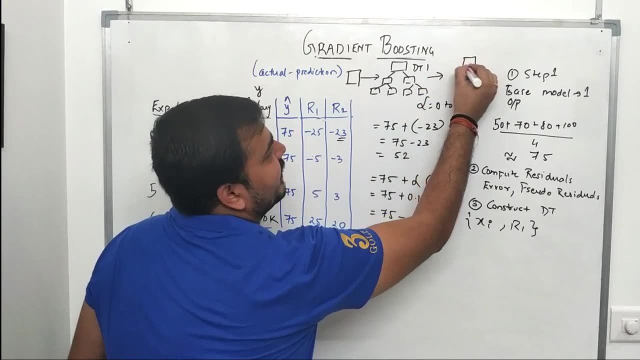 Okay, so here I've got my value 73. But still, this value is having a huge difference, right, When compared to the output salary. So what we'll do after this? we will add one more decision tree Now. this decision tree will be now created based on the output value. So the output. 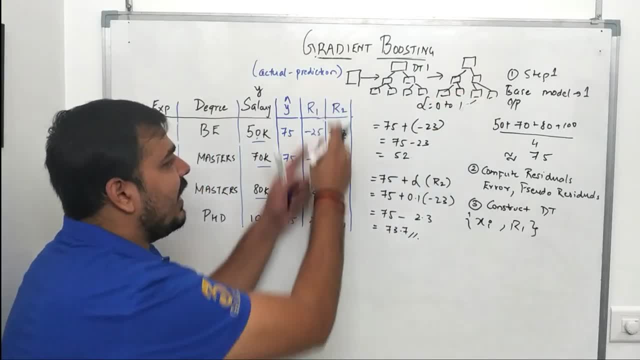 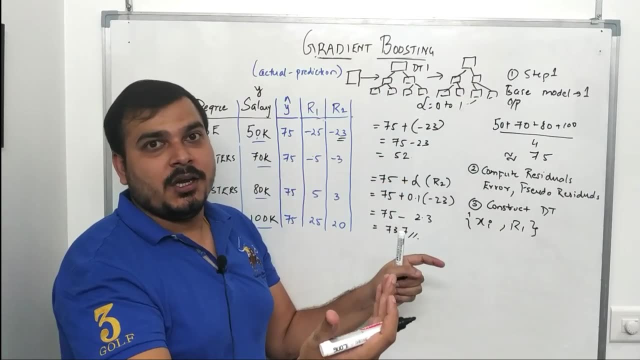 output based on the output of this R2 value, that is my residual 2 value, and my independent feature will be same. So this decision tree will be computing my next residuals. Okay, one after the other. So what I can do is that I can write a generic formula saying that f of X is equal to my base model. 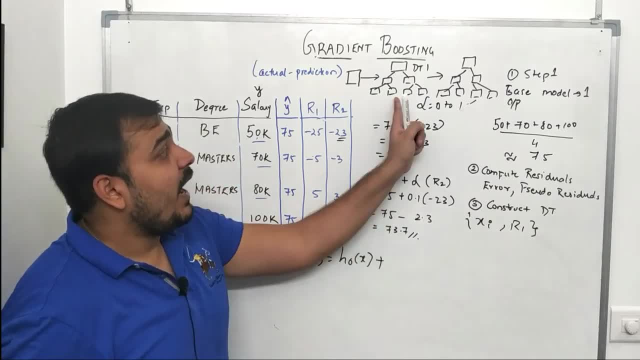 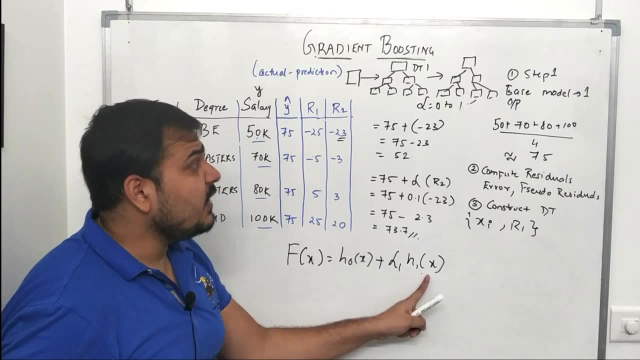 I'll write it as H0 of X Right Now. if I want to add one more decision tree, this will become alpha 1, H1 of X. H1 of X is nothing, but I understand the output that is given by this Right. Similarly, if I want to add one more, 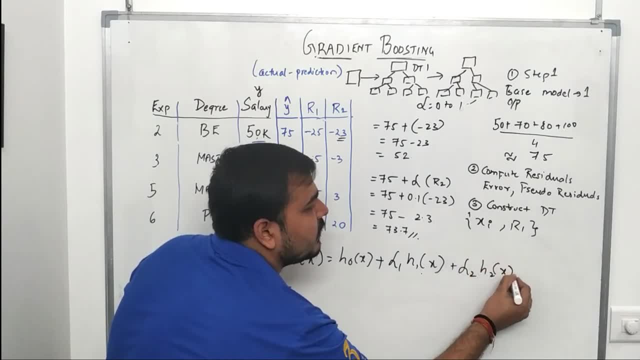 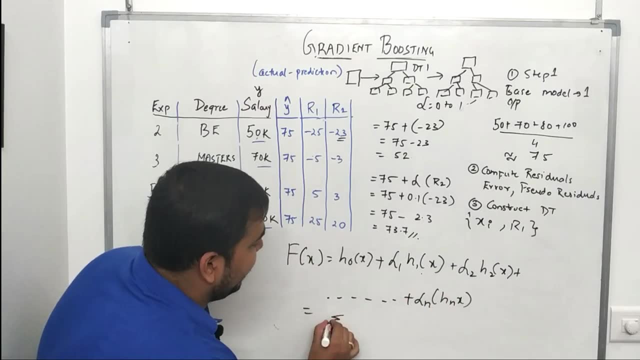 decision tree. then it will become H2 of X. Similarly, like this, I will be having alpha n Hn of X And finally I can write it as sigma: i is equal to 1 to n H of i. Sorry, alpha of i H of i X. 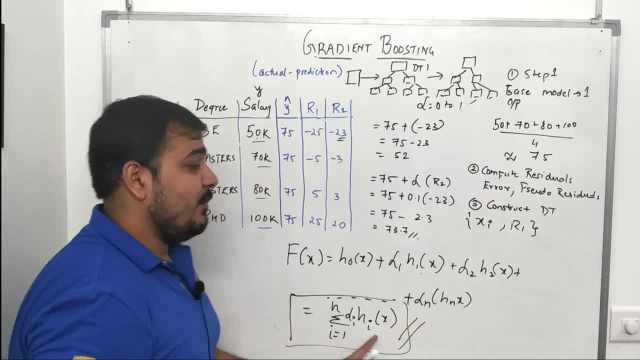 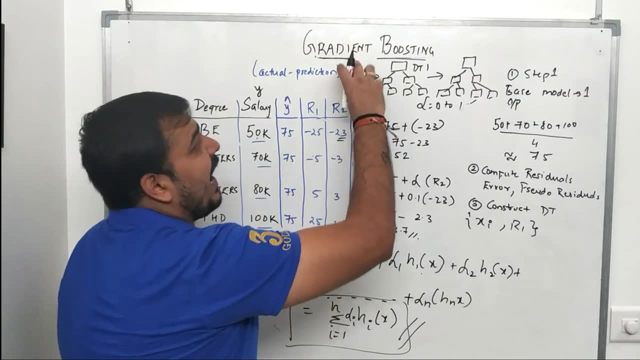 Right. So this is my final output And again, I'll be discussing about this in more depth In my pseudo algorithm. that is my next video, But just understand what we are doing. We are adding after one base model, we are adding, we are creating this sequential decision tree. 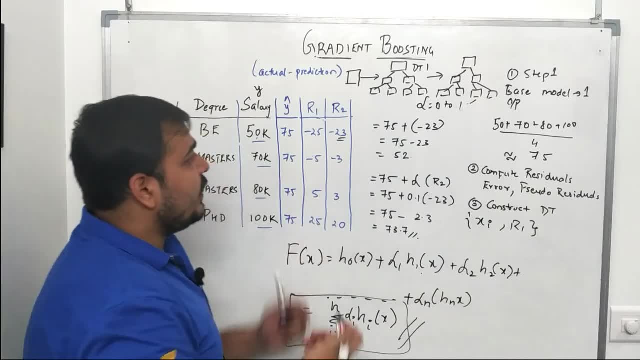 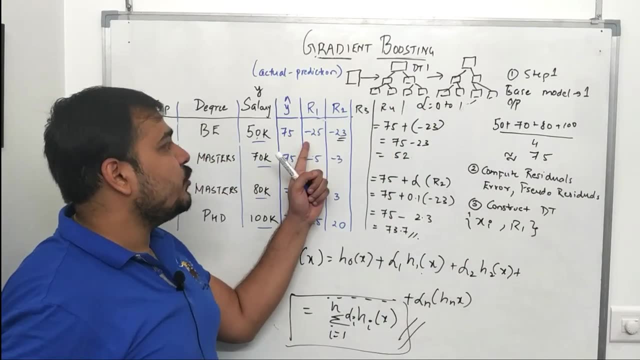 based on this residuals that we are getting, And by that you'll be seeing that after some time this residual will also be decreasing. This residual will also be decreasing this value. You can see that minus 25,, minus 23,. then minus 20,, minus 19,, minus 18.. 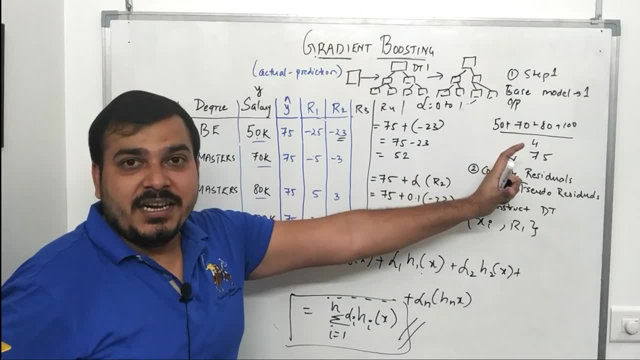 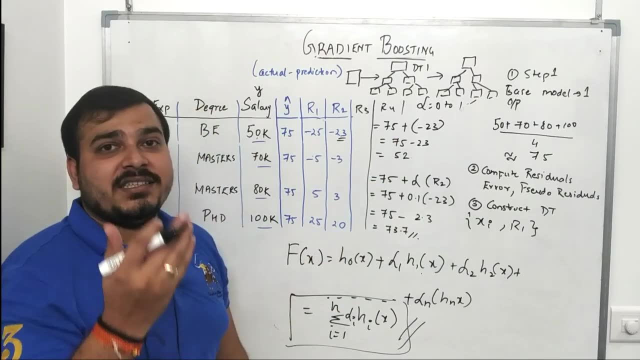 So like that, minus 15,, minus 10,, up till some decision tree will be going, And this our main aim is to basically to reduce this residual error And after that, suppose, any new test data that comes we have to pass. 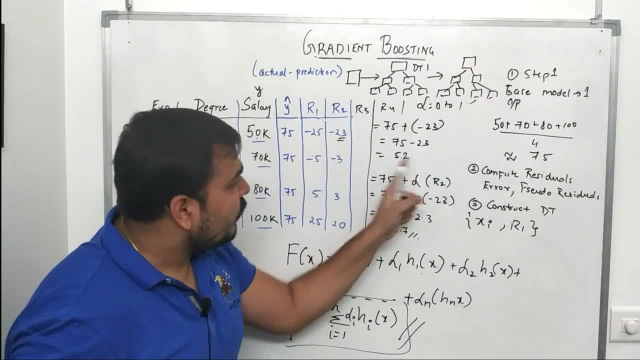 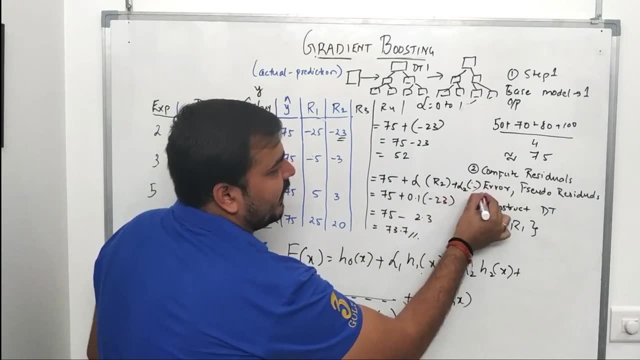 from this base model to that many decision trees And we need to try to add this in this way. So suppose one more decision tree is there, I'll be adding with alpha 2 with my next H of X, then alpha 3 with my next H of X. Like that I'll be continuously adding. you know it may be a minus value. 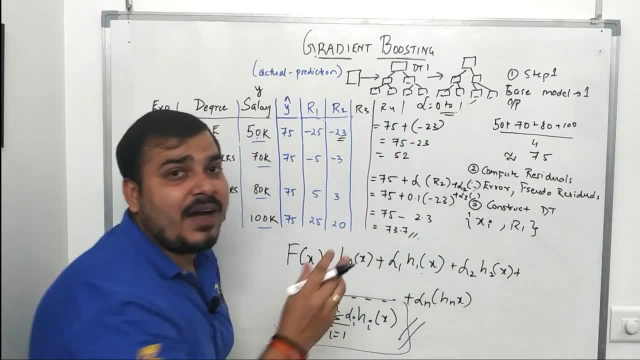 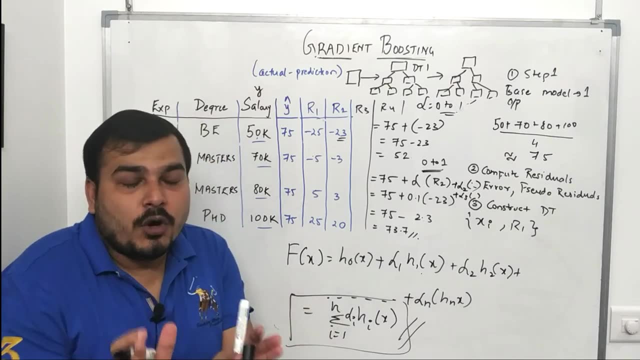 It may be a plus value, And this alpha value you usually decide with the help of hyperparameter tuning Right. It will be again between 0 and 0.. Now I have got- I hope you have got- the idea, guys, how a gradient boosting works. 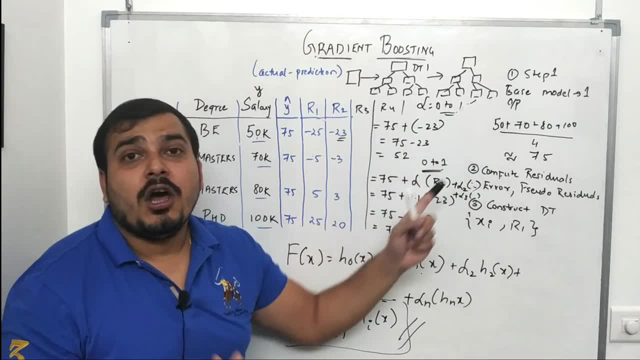 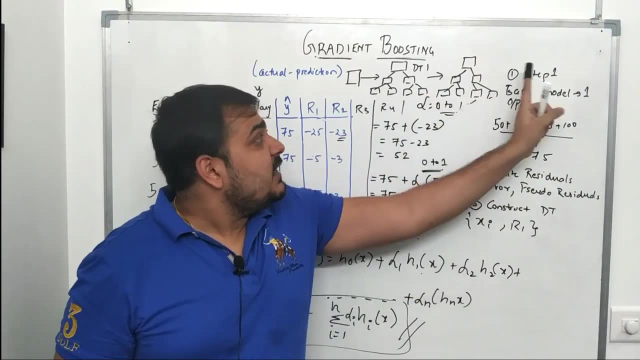 Why we call it as a sequential tree. Why we call it as a boosting tree? Because understand, after the base model, we are adding decision tree sequentially. We are adding sequentially, Right, We are boosting this base model as we go ahead with the help of this residual values. 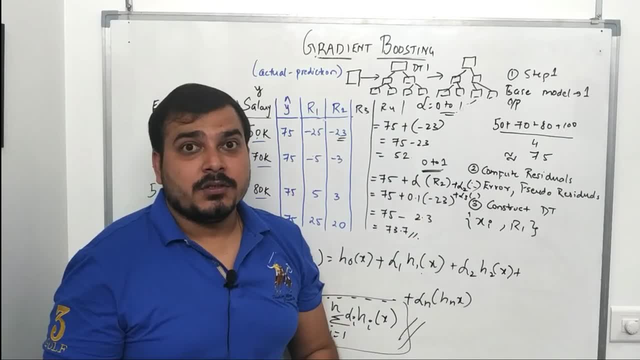 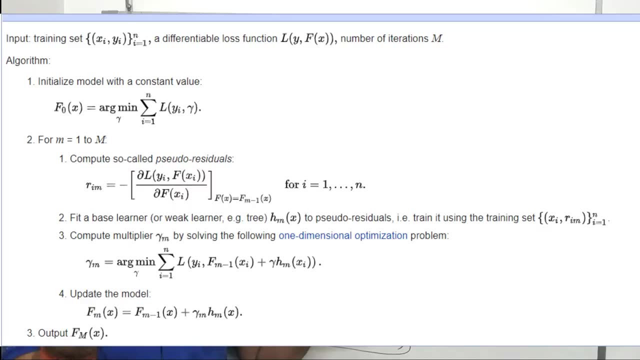 that are getting computed. that are getting computed, So I hope you understood this particular video. Now, guys, in my next video, I'll be discussing about this pseudo algorithm And, if you want to get a head start, I'll be giving the link of the Wikipedia in my description of this particular video. 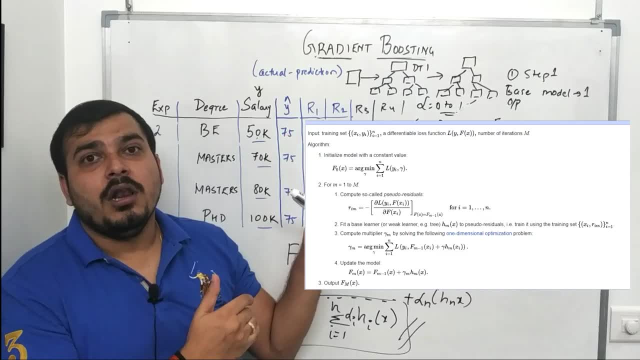 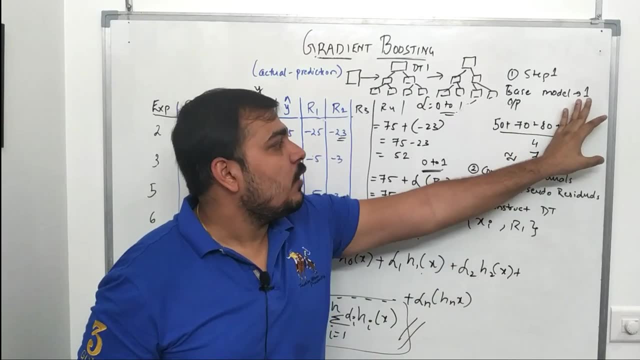 Just go over there have a look. This is how the whole gradient boosting actually works And that I'll try to discuss mathematically, Like: how do we come up with this particular base model? How do we calculate the average value, How do we compute the residual values, Everything.